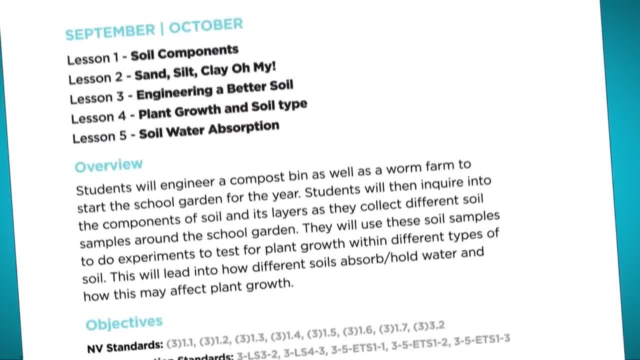 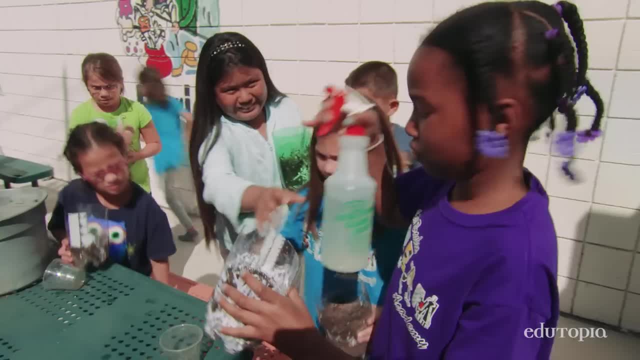 We went through the Nevada State Standards and the Next Generation Standards and we wrote curriculum based on that. You'll see the art teacher out there with the kids. There's math, science, there's everything When they're working in the gardens. it's all tied to our standards. 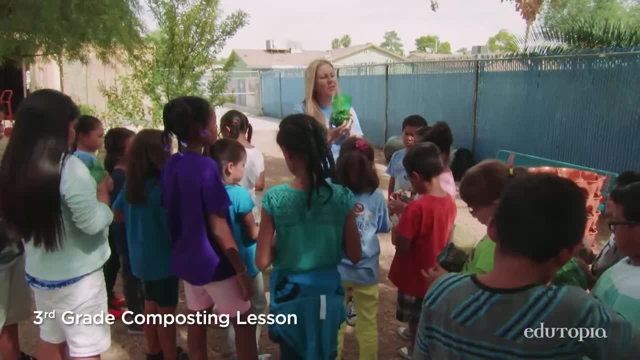 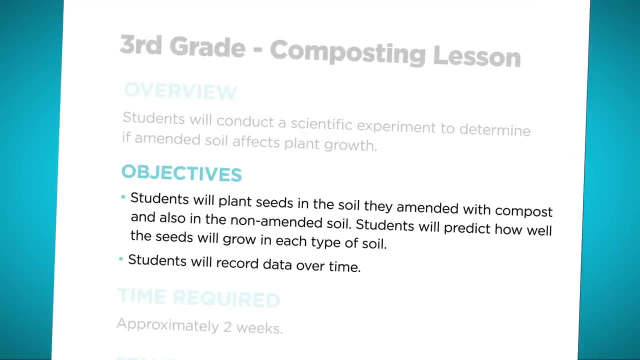 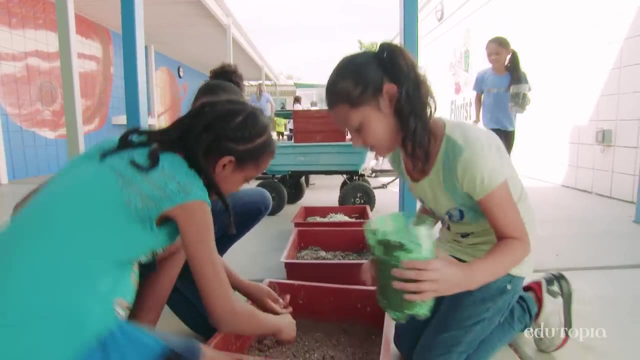 We want to be able to feed our worms and we want to be able to add to our compost. We typically do a garden lesson at least two to three times a month. Part of our science curriculum is looking at plants and nature, So we thought it was a great asset for students to learn how they can reuse scraps and soil and worms to help make our soil better. 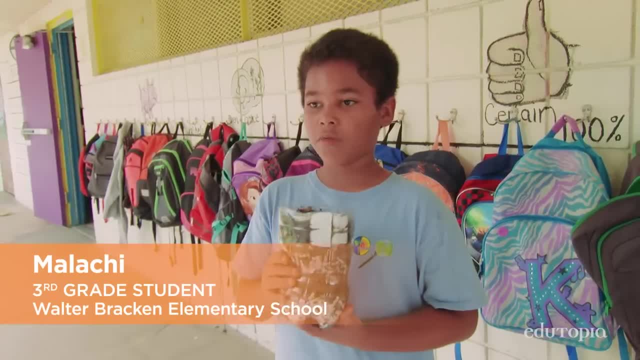 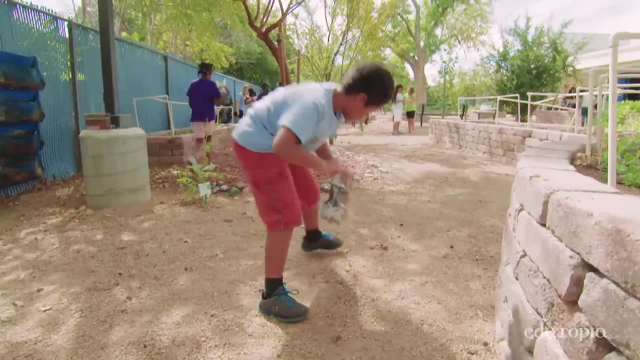 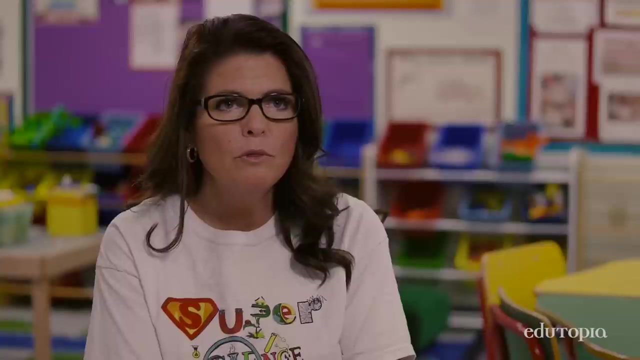 An organic thing is something that humans eat and then they throw away, but they can actually put it in a compost or in the dirt. I think this is more important than math and science, because you're helping nature grow Initially. I just wanted my students to know that vegetables don't come from the grocery store. 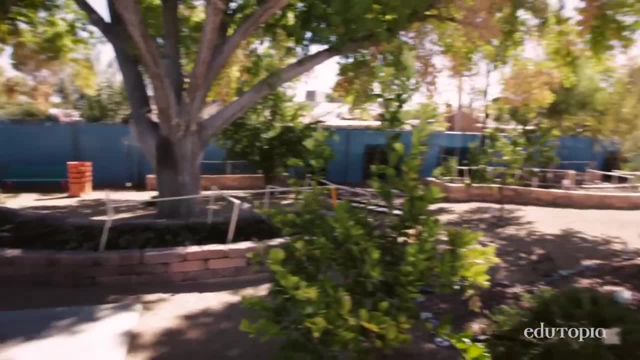 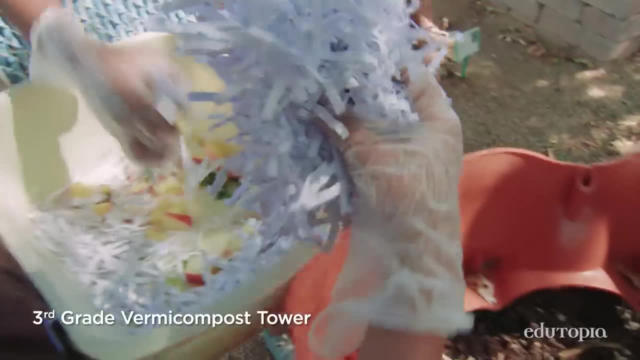 They come from the soil, from the ground They grow, and it's a process, And to do a lesson once in a classroom with a lima bean in the window is not enough. We're checking in If the worms they pooped or they peed. we check it by this. 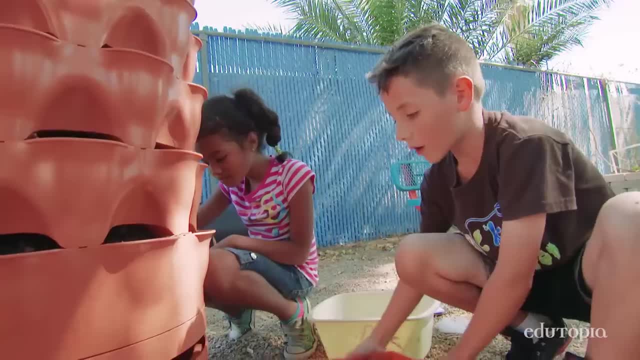 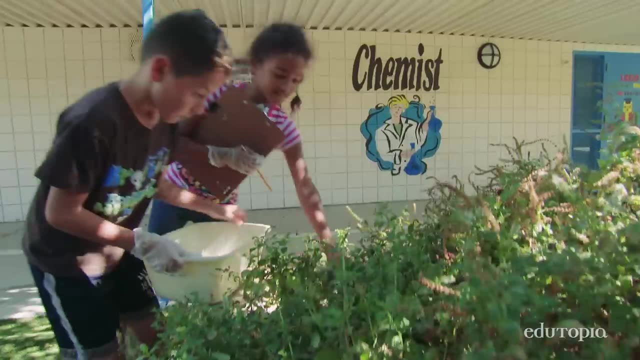 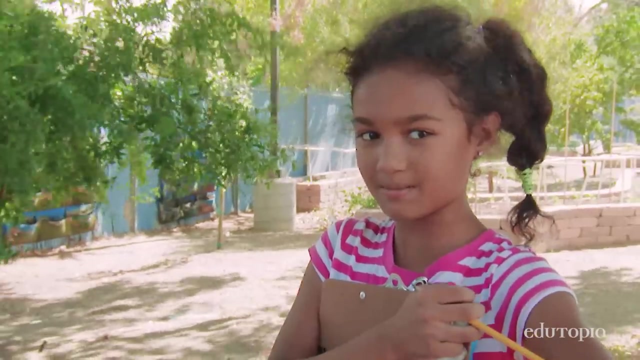 We need to pee so we can water our flowers and make them grow more. Students are actually in the gardens every day, even if it's only briefly So. sometimes it's something just a 10 minute activity where they're maintaining. I check to see if the soil is moist by dipping my finger in. 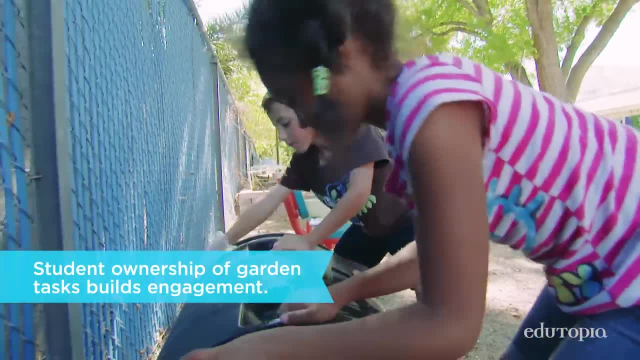 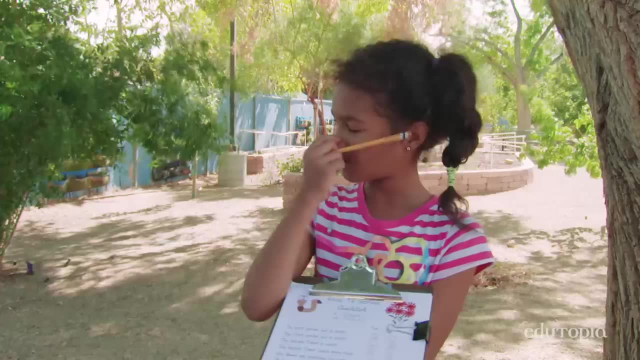 The last thing I have to do is turn the compost bins around. I got to see if it's moist, I see if there's any problems, and if there is, I check off yes, and then write it down here. I think one day maybe I'll have a garden of my own. 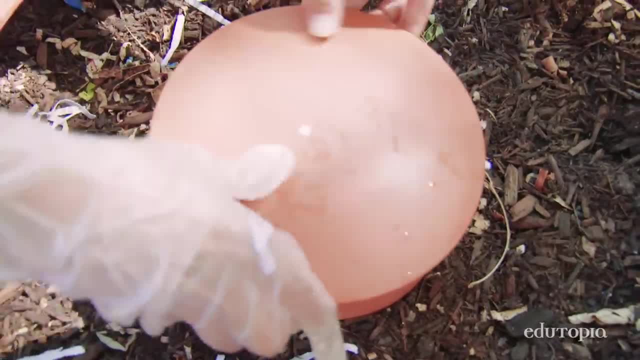 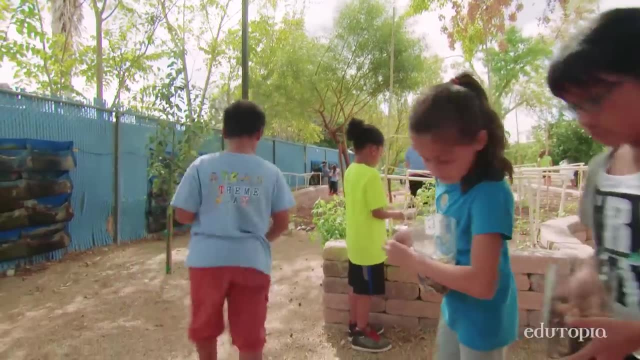 It might look like they're running around, but they're really not. They have very specific jobs and they're planting and they're harvesting and they're checking for bugs and they're collecting seeds. They're planting farmer's markets so that we can sell the produce and make money to fund the gardens.